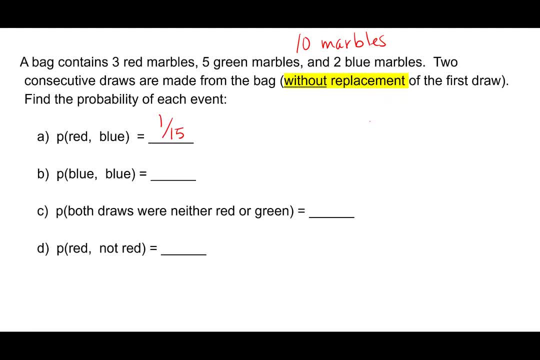 says: what is the probability that the first marble will be blue? Leave that one out and the second marble will be blue. Okay, for the first marble to be blue, there's two blue marbles at the very beginning, out of a total of 10 marbles. We're going to multiply that by the fraction. Let's think about. 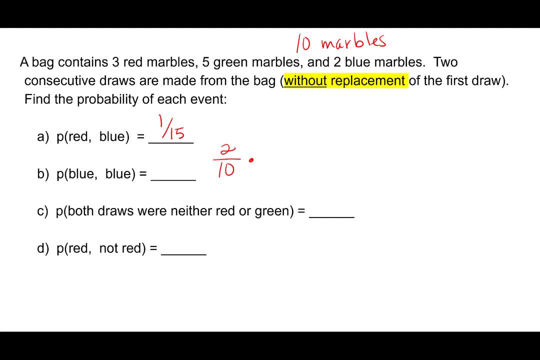 this. We already took a blue away from the bag and so we know from the previous problem the denominator will be out of nine Marbles. but do you see that, because it was specifically a blue, we no longer have two blue marbles in the bag, We only have one. so my numerator will be one. Multiply that straight. 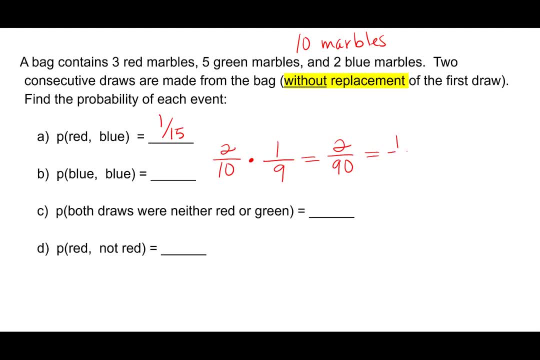 across to get 2 over 90 and then simplify that to the fraction 1 over 45.. Okay, take a look at the next question. It says what is the probability that both draws were neither red or green. So if the marbles were not red or green, that means they're blue. which bad, Miss Cornette. 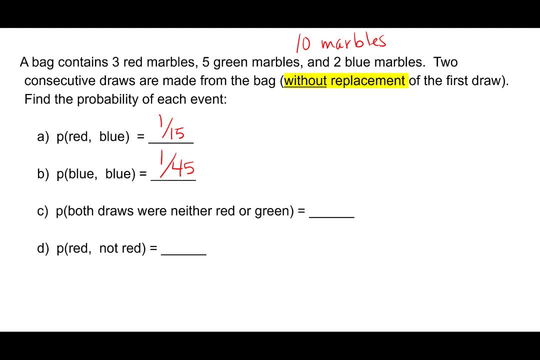 this would be the same question as the one we just talked about, So let me just, in the middle of the video, let me change it up. I'm gonna cross out or the or green part. So let me read it to you again: What's the probability that both draws were not red? Okay, so what does that mean? that they? 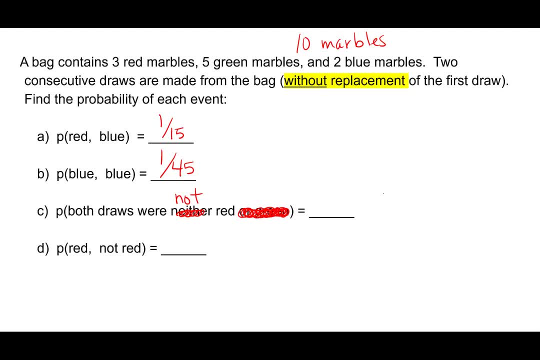 could be blue or green. Okay, so draw number one. we know we're going to have 10 marbles. We can pick either a blue or a green. There's five green and two blue, So there's seven non red marbles in the bag. Okay, we're. 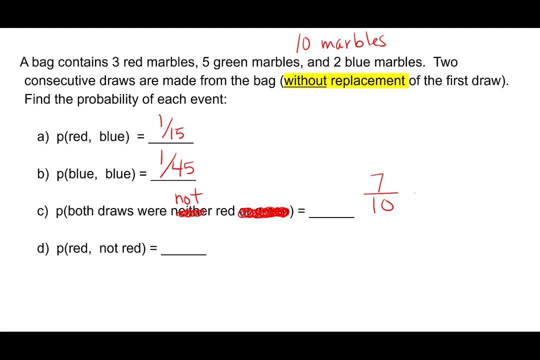 going to keep that non red marble out And we're going to now go in and draw a second time. Because that non red marble is out, there's only a total of nine, So that goes in our denominator, And because it's a non red marble, we don't know if it's green or blue.